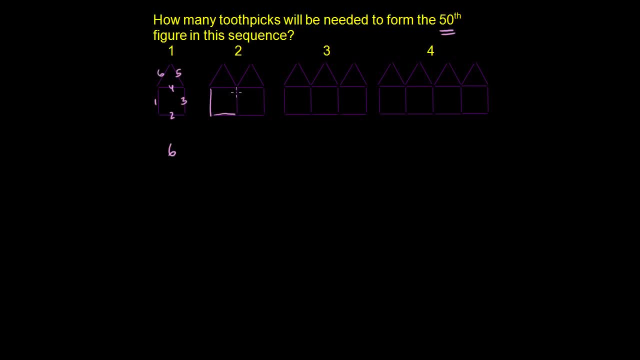 first right. This is the first figure right here. Let me just trace it. That's the first figure right there. And then, how many new toothpicks are we going to have? We have one, two, three, four, five. 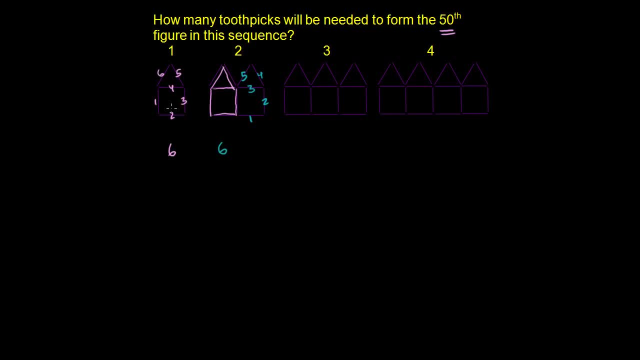 So we have six plus another five. So we have the six in the original one plus another five, which is equal to 11 toothpicks. Now what happens in this third object, Or this third little toothpick house-looking drawing thing? So we have our figure from the two houses. 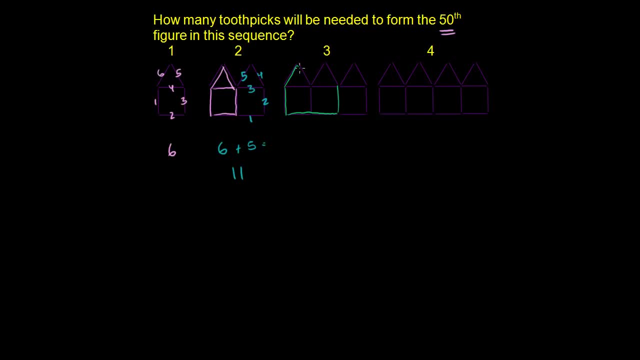 So we have those right there. This is the exact same thing that we had as our second object. So that's that right there. And how many more do we have? Well, it's going to be the same thing. We've just added on this other extension to our house. 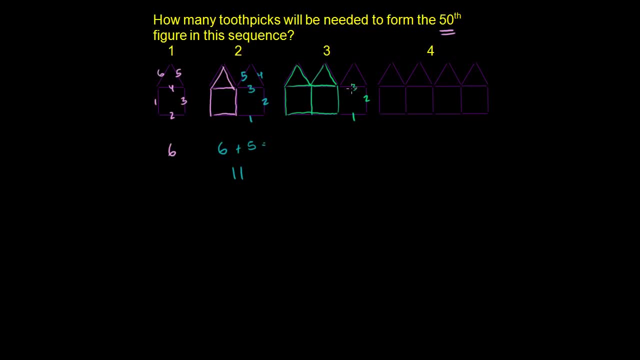 You can view it that way. So we have one, two, three, four, five. So it looks like every time we go down this sequence we're adding a new object to the sequence, We're adding five toothpicks. So here we're going to have 11 plus five. 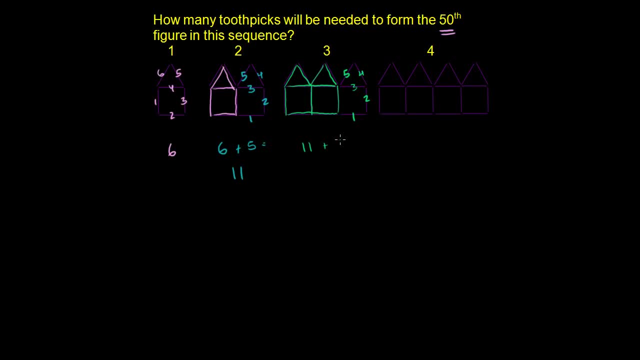 There's 11 toothpicks in this part of it And then we have another five, 11 plus five, which is 16.. Same thing over here. We have 16 in this part of the drawing. That part of the drawing is going to be 16 toothpicks if. 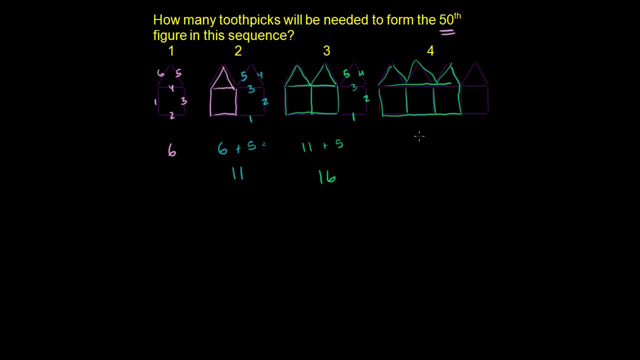 you draw all of that And then we're going to have another five right here. So this is going to be 16 plus five Or 21.. So how can we figure out how many toothpicks we're going to have in the 50th figure? 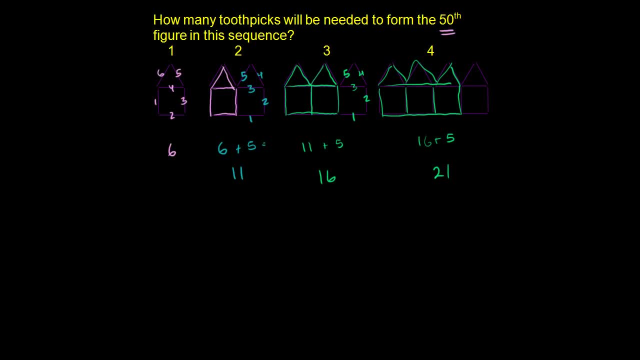 I mean, we could draw 50 of them, but it's going to take us forever. So all we have to do is realize the pattern: Every one. we're just going to add five, Or we can even come up with a formula for the nth figure. 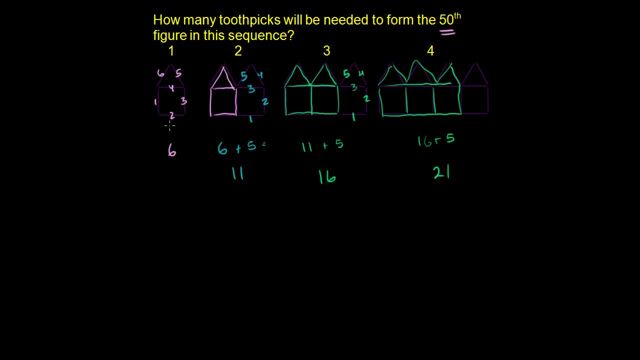 How many toothpicks in the nth figure. So here in the first figure we have, you can view it this way: in this first figure we have one plus five toothpicks. We have this one. You can imagine that was always there, and then you: 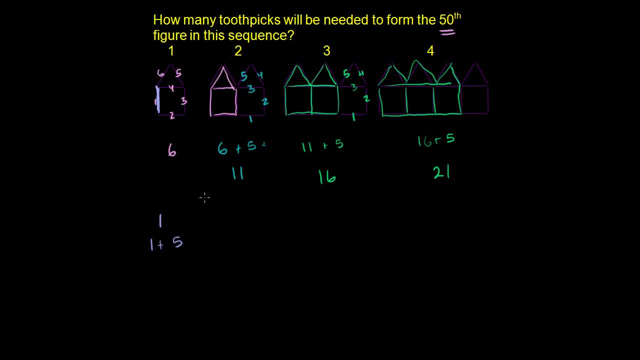 added five right there. So that's our first term in our sequence. Our second term in our sequence, what do we have? We have six, which is one plus five. So we have that one plus five plus another five, Plus this five right here, plus another five. 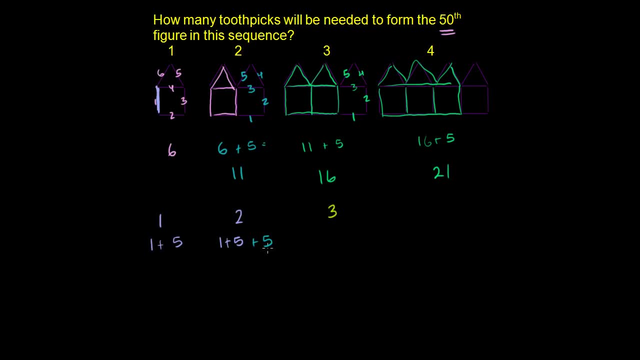 And then our third term, in our sequence. what do we have? We have all of this business that we had in the second term, so one plus five plus five, And then we have another five. We do it in green. We have another five. 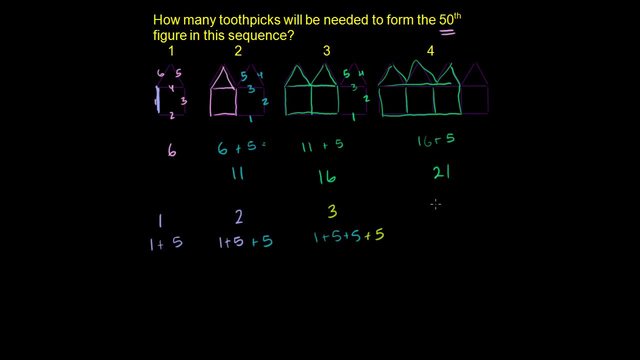 And then, finally, in this fourth term, what do we have? So in the fourth one we have everything that we had in the third figure, so one plus five plus five plus five, And then we add another five, We add a fourth five. 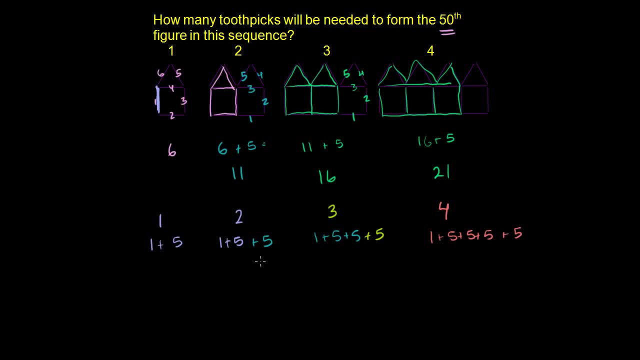 We add a fourth five right there. So why did I do it this way? Because I wrote this first one as one plus five instead of just a six. because you can see, well, look, I had a one and then I had one five. 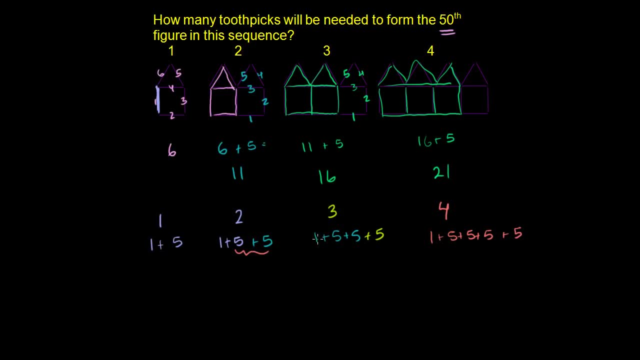 Now I have a one and I have two. I have two fives. Now I have a one and I have three fives. Now I have a one and I have four fives. So you might see the pattern. If I had the nth term right here, I will have a one plus. 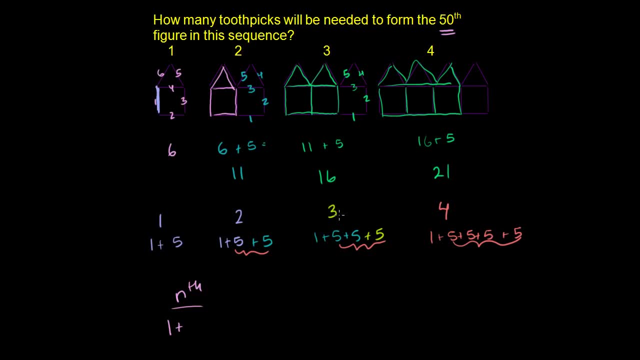 n fives, right, The first term has one five. The second term has two fives. Third term has three fives. Fourth term has four fives. So the nth term, If this is 10, it's going to be one plus 10 fives. 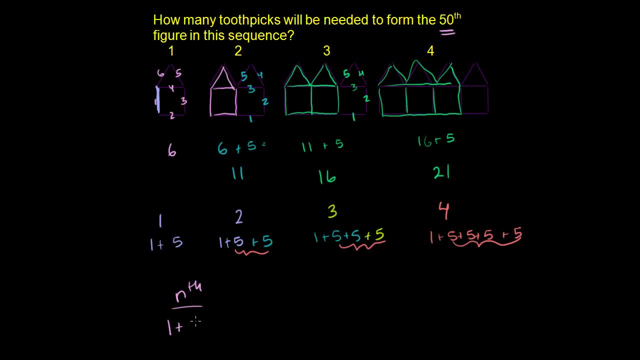 Or if it's n. if I'm kind of abstracting a little bit, I'm going to have one plus five times n. right, And try it out. If n is equal to one, it's going to be five times one. 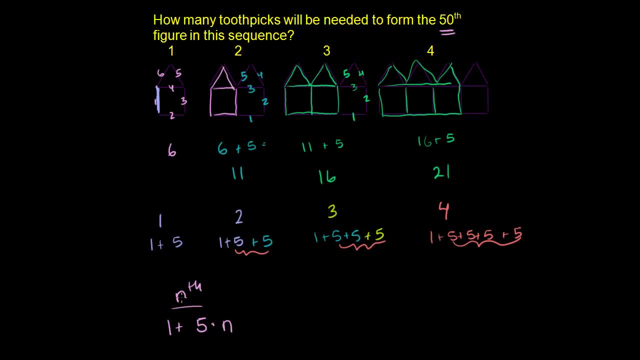 If n is equal to two, it's going to be five times two. If n is equal to three, it's going to be five times three, So that when the 50th term, if we're talking about the 50th term, 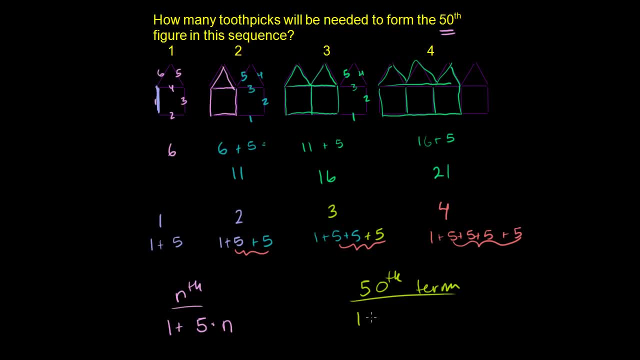 What's? how many toothpicks are we going to have? We're going to have one plus five times 50, right n is 50 here, which is equal to what? Five times 50 is 250.. That's 250.. 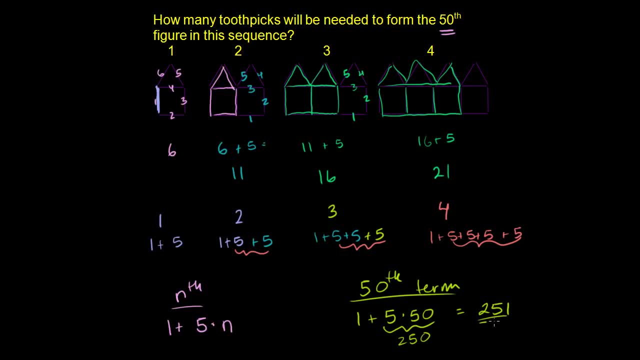 And then we add one. We're going to have 251 toothpicks will be needed to form the 50th figure in this sequence.